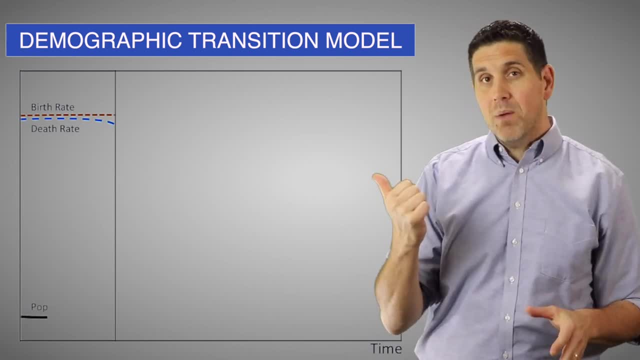 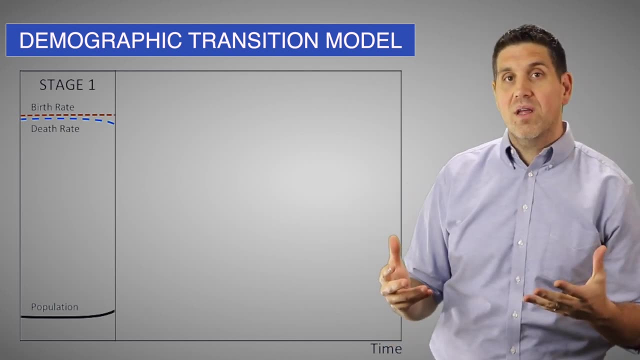 food for themselves, not to sell, And the result was that global human populations stayed relatively low for thousands of years. This is stage one of the DMT, and it's the life of the vast majority of the people who've ever existed. Oh, that's depressing, But over time, people started to grow. 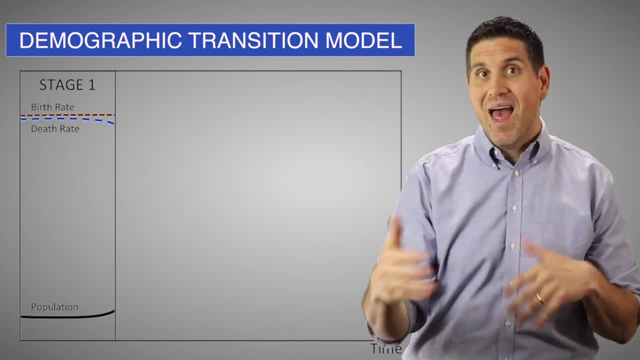 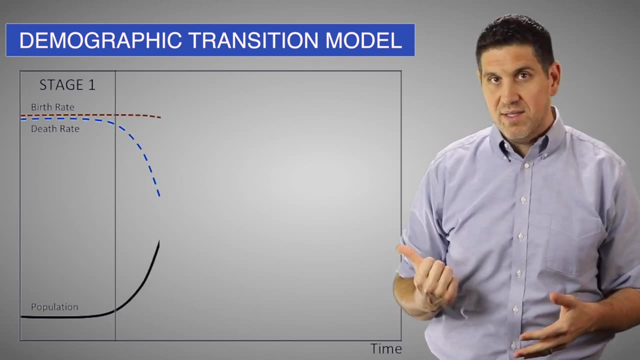 more food, and that was not just for themselves, it was for other people to sell it, and that created agricultural-based economies. And more food means less famine and higher living standards, so the death rate started to decrease, And at this point people started to grow more food and that 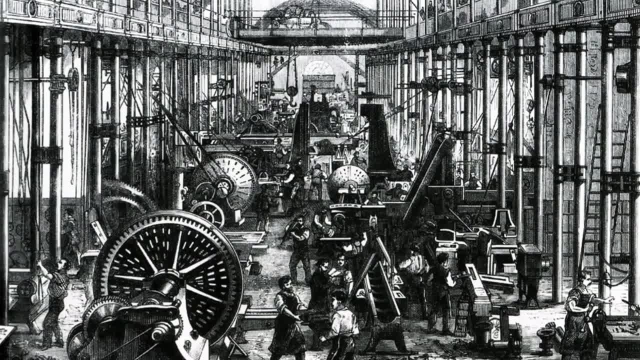 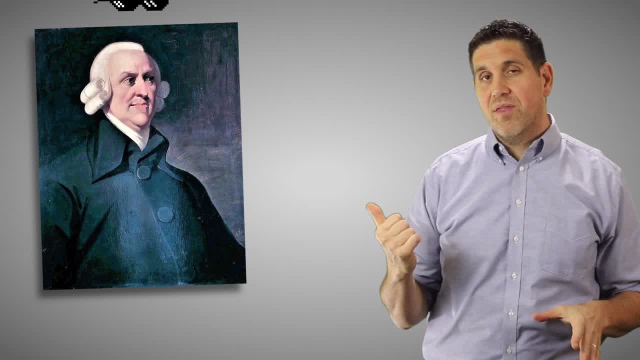 led to the industrial revolution. Technological advancements like the widespread use of the steam engine, changed what would be produced and how it would be produced. It's also when Adam Smith, the founder of modern economics, wrote about how markets and economies work, and when Thomas 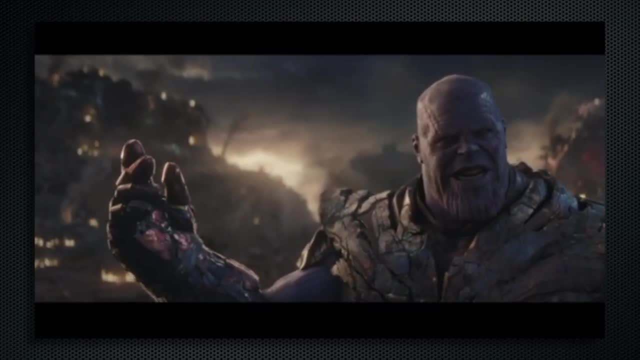 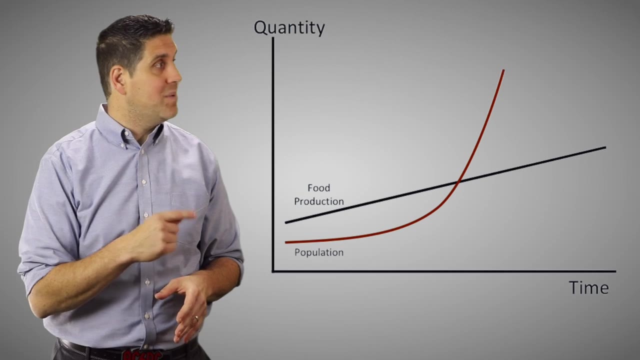 Malthus wrote that we're all going to die of starvation. I am inevitable. Malthus noticed that our ability to produce food grew at a linear rate, but population grew exponentially, And his logical conclusion was that eventually we're going to run out of food and 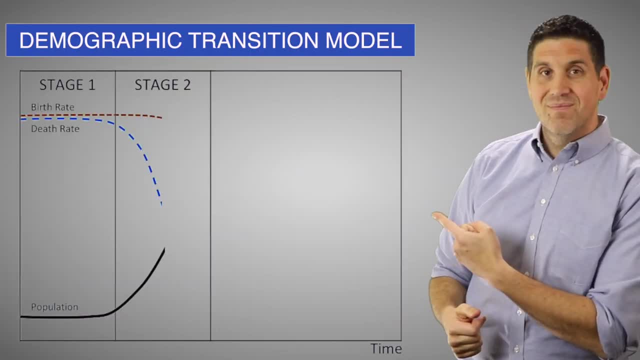 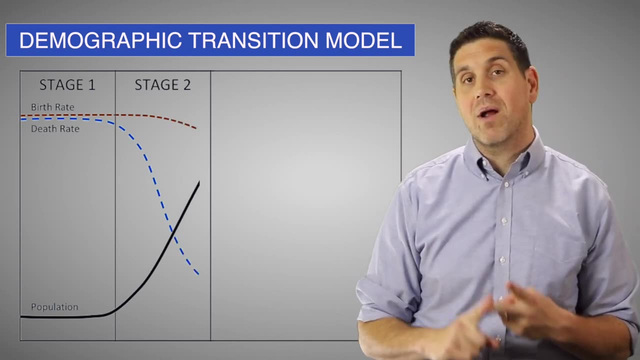 people are going to starve And the DMT shows that he was right. kind of Population here in stage two is increasing at an increasing rate but industrialization brought new technologies and more productivity. that led to more food production And industrialization led to better 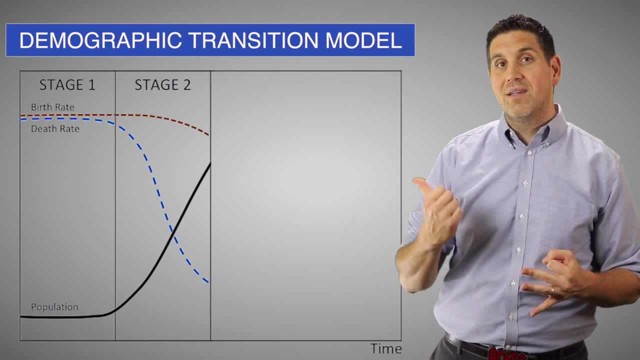 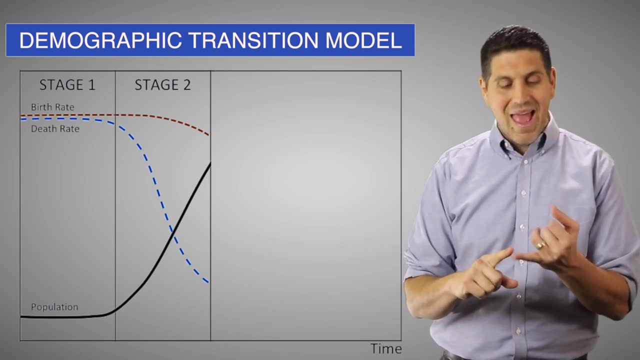 healthcare, education and sanitation, which decreased the death rate. But notice that the birth rate didn't really start to fall because a lot of families felt an economic need to have more kids to farm the land and they didn't realize that a lot of their children are. 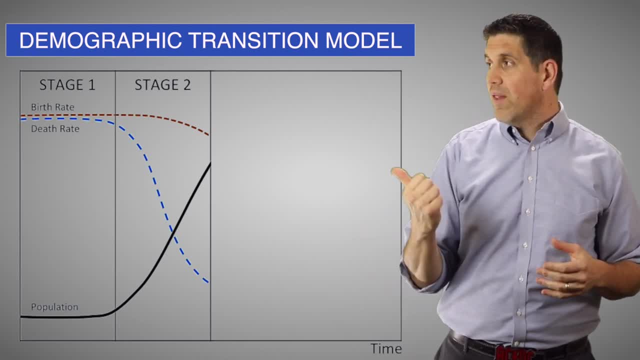 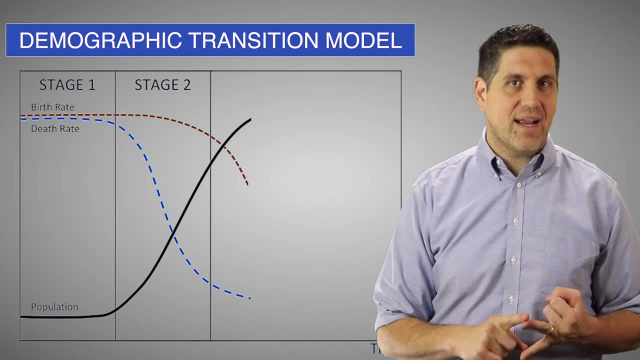 going to reach adulthood. In other words, they didn't know that the death rate was falling. so they continue to have a lot of kids, And as economies industrialize, people move from rural to urban areas, from farms to factories. This means that a lot of families didn't have either. 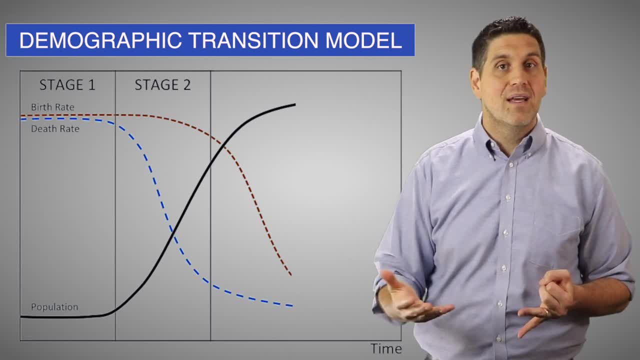 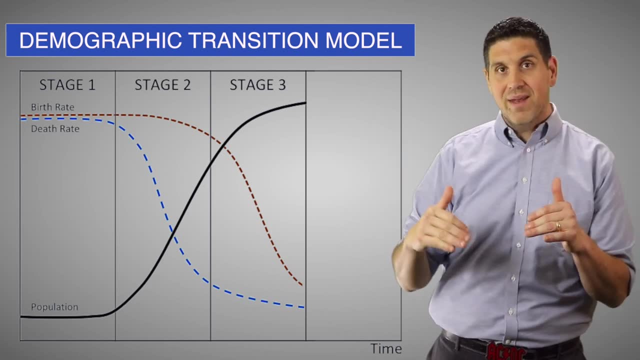 the room or the necessity for a lot of kids, and so the birth rate started to fall. This is stage three, when the population is increasing, but at a decreasing rate, because the fertility rate has fallen and people are having less kids, And advancements in production and trade led to. 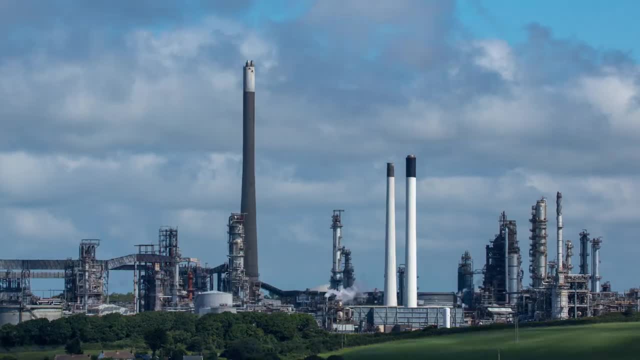 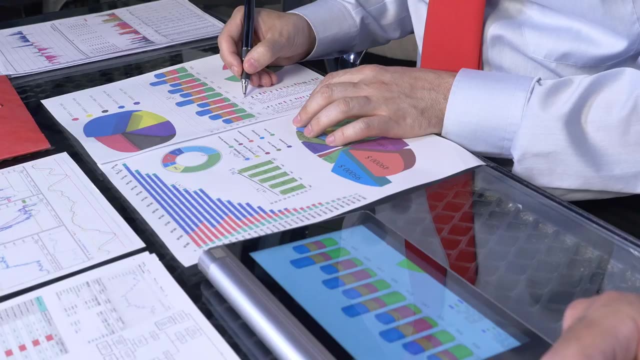 higher living standards and a decrease in extreme poverty. This is the world of industrialized countries. Now, here in stage four, we have post-industrial economies where the focus isn't on manufacturing, it's on service industries like finance, insurance and healthcare, Birth rates and 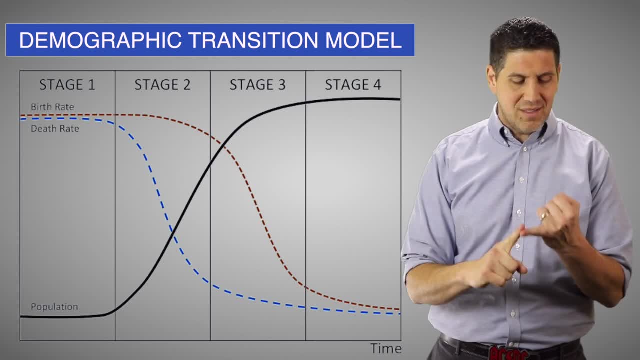 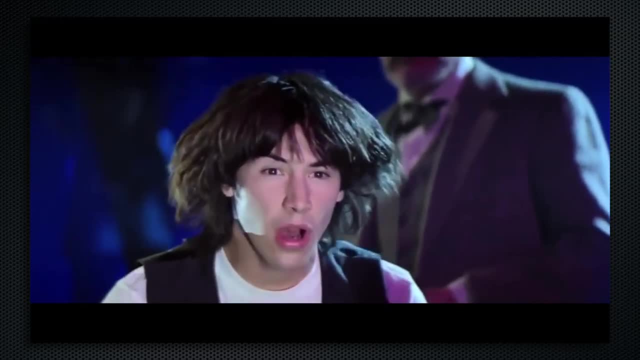 death rates are low, so there's zero population growth, and life expectancy, gender equality and living standards are the highest they've ever been in the history of the world. Whoa Now, up to this point, I've been talking about Western industrialized countries. 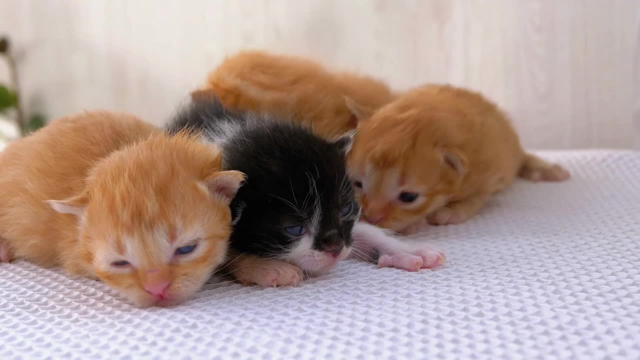 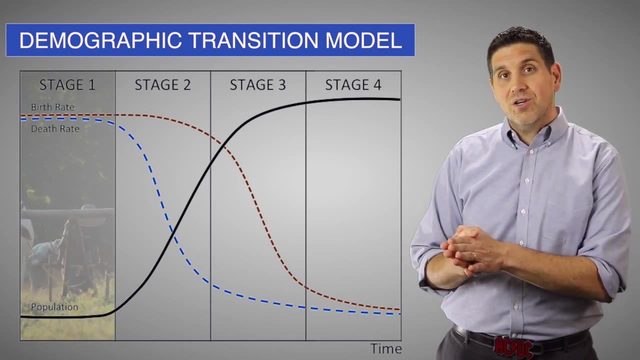 but this process is happening all over the world. Every country is at a different stage of development. You can see that in their demographics. Right now there's really no countries that are in stage one, but there are some countries that are in stage two. 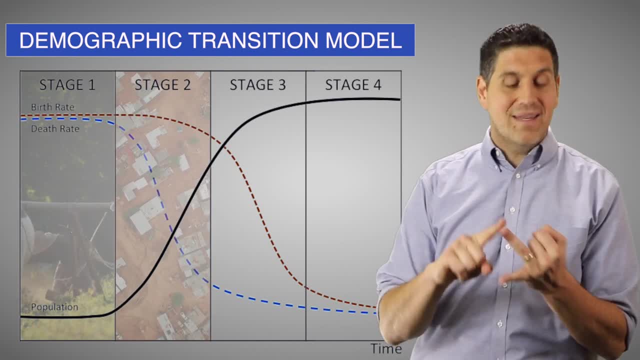 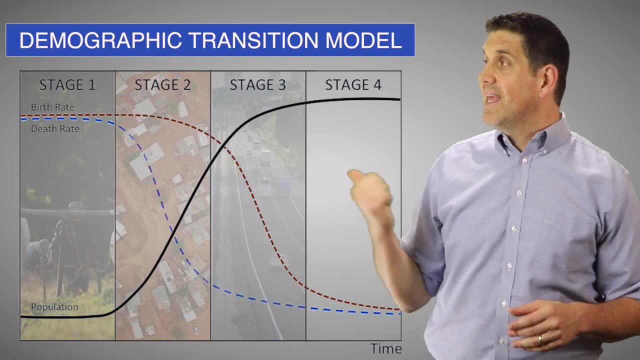 These countries have underdeveloped economies so they have high birth rates and high death rates and population growth that's exponential. These are countries like Angola, the Sudan and Guatemala, And other countries like India and Mexico are already at stage three where people have already moved into factories and they have falling birth rates and they have 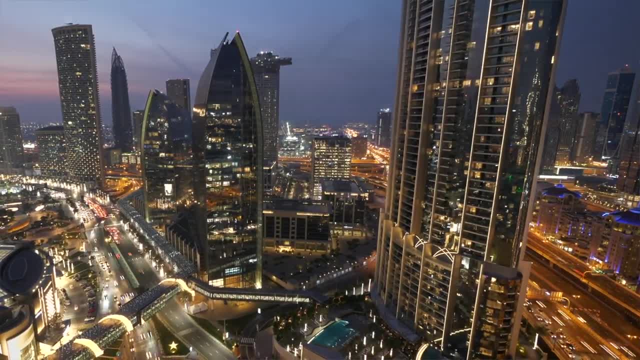 higher standards of living, And countries like China and Canada and the United States are at stage four with very little population growth, And that's why we're talking about the post-industrial world. And there's also a theoretical stage five with countries like Germany and Japan. 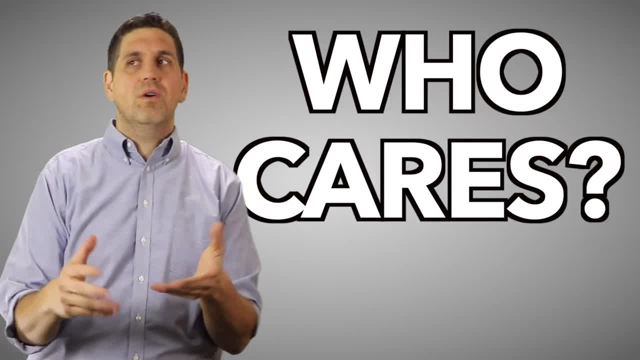 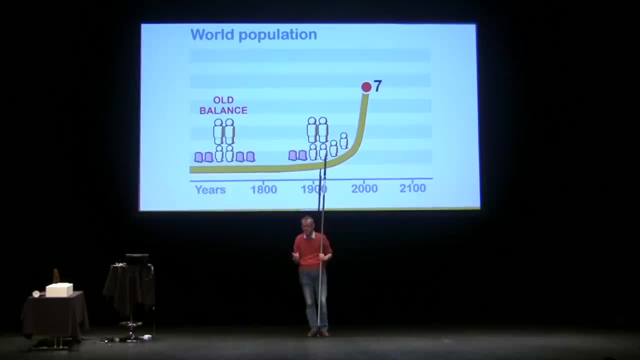 where the population is actually falling. Okay, so who cares? You do, because it's important to understand economic development, so you don't have preconceived ideas about the world. But there's so much crap written and said about population growth. There's people out there that are pushing the government to do things to limit population growth. 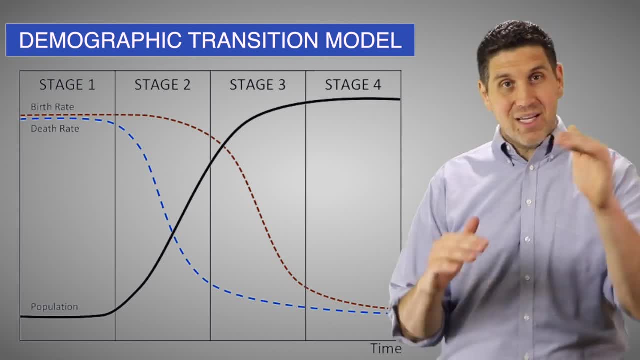 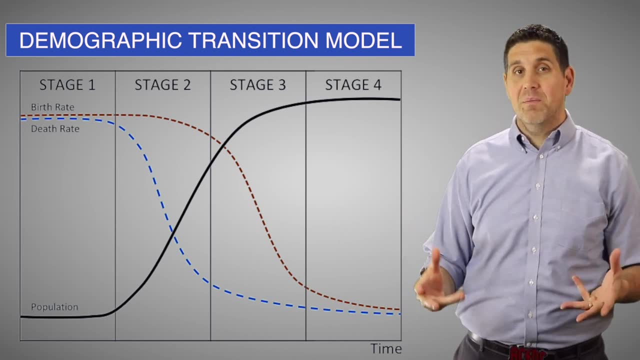 but the DMT shows that population is going to level off anyway. It's going to cap out at around 10 or 11 billion sometime in the next 50 years. But that creates a whole set of new problems. Right now, the richest 10% of humans account for about 50%. 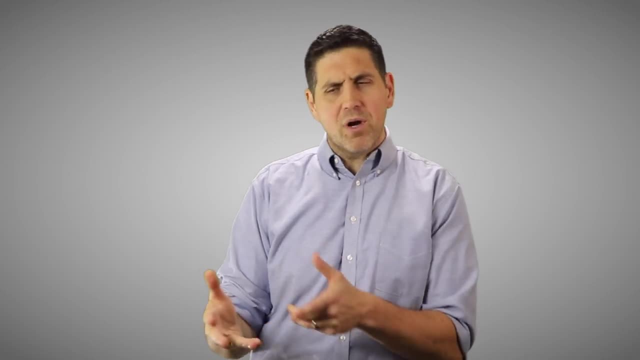 of the world's CO2 emissions. As more and more countries develop, the people are going to want more things, and that's likely going to put a strain on our resources and the environment. And if you think about it that way, the problem isn't. 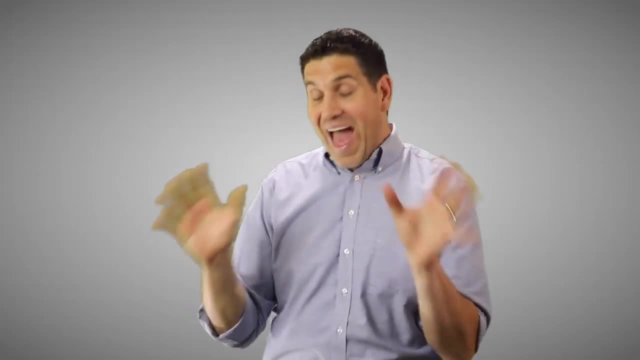 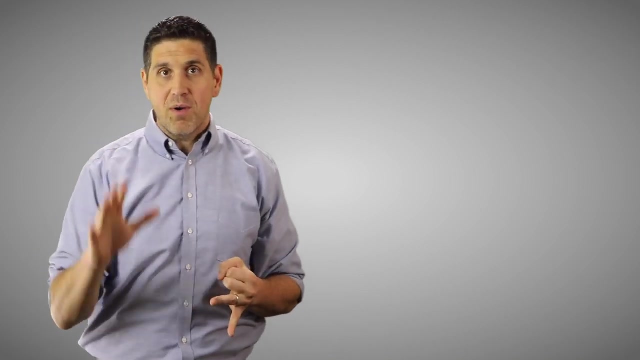 are there too many people? It might be. are there too many rich people? But that is a whole other video. Hey, thank you so much for watching. If you're a student in economics or a human geography class, take a look at the ultimate review packet. It's going to help you learn and study and